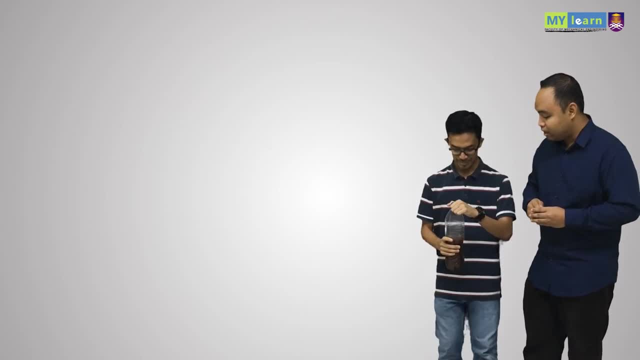 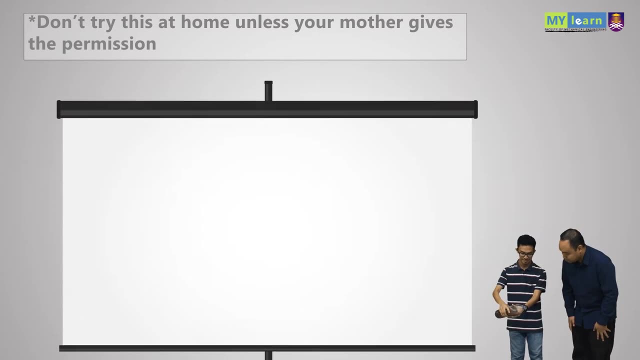 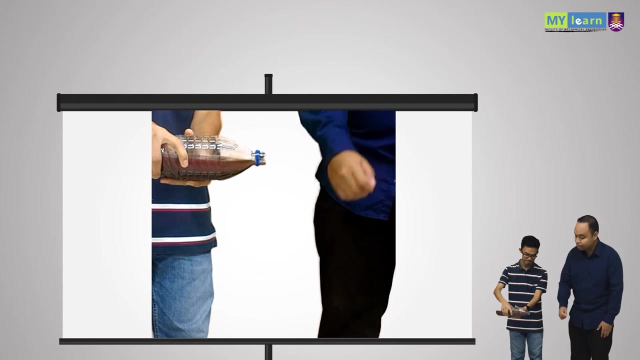 a simple example of laminar and turbulent flow. Can you keep it stable and make sure the water goes into the dustbin? Okay, try it. Okay, so what you see right now is colored water inside the bottle and we are trying to flow the water down into the dustbin. So you can see from here the turbulent flow. 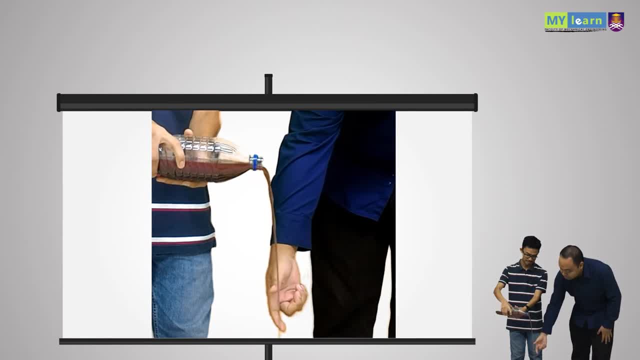 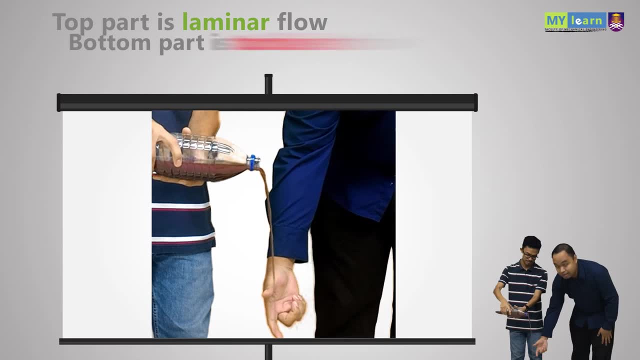 is actually a laminar flow, while the bottom part of the flow is low in velocity while the bottom part is high in velocity. So the top part of the system is actually a laminar flow, while the bottom part is a turbulent flow. So somewhere in between we will have 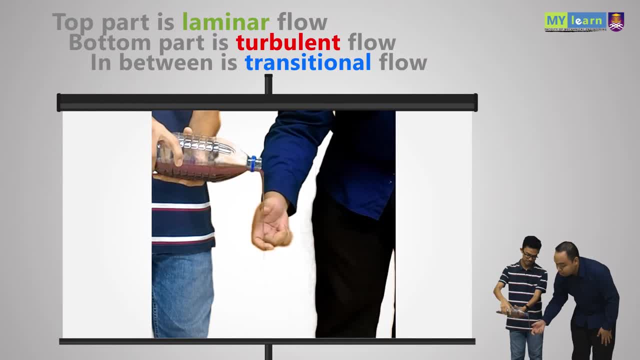 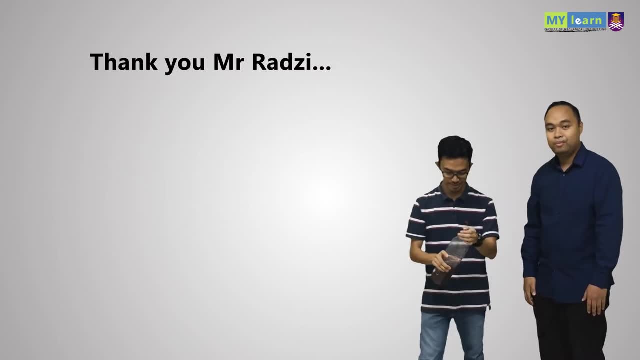 some laminar and some turbulent, and this transitional flow will be the one connecting between laminar and turbulent flow. Thank you very much, Mr Razid. And after this, we will show you how to calculate the Reynolds number. and through the Reynolds: 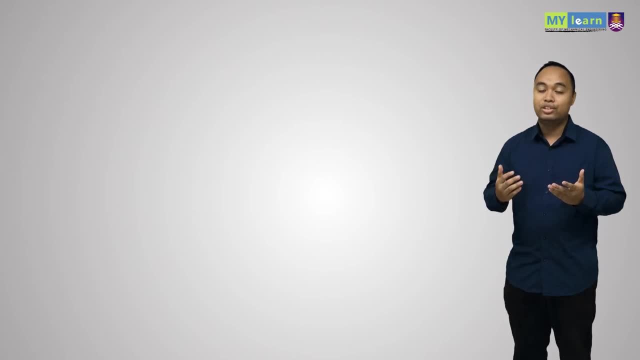 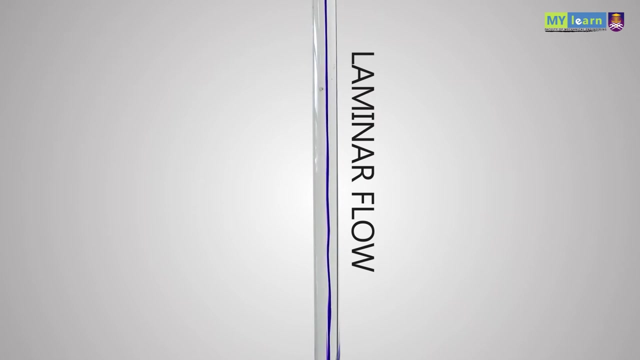 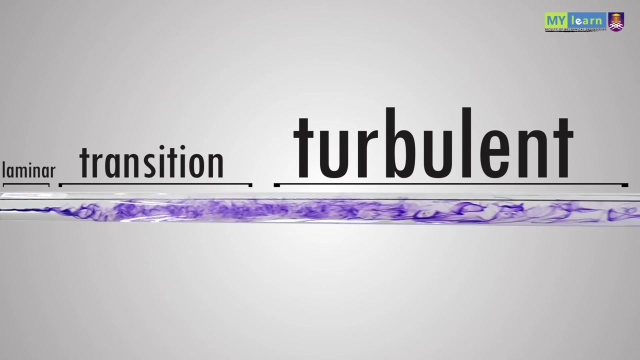 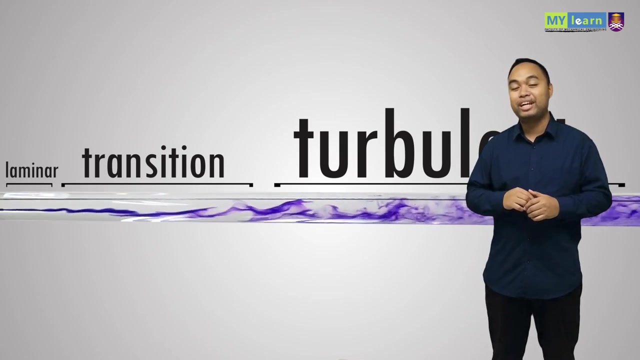 number, we can know whether it is a laminar flow or a transitional flow, or is it a turbulent flow. So till then, bye. flow through visualization. So there is another way to find out whether the flow is laminar. 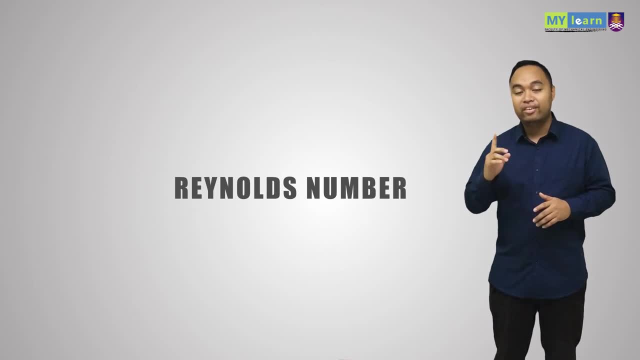 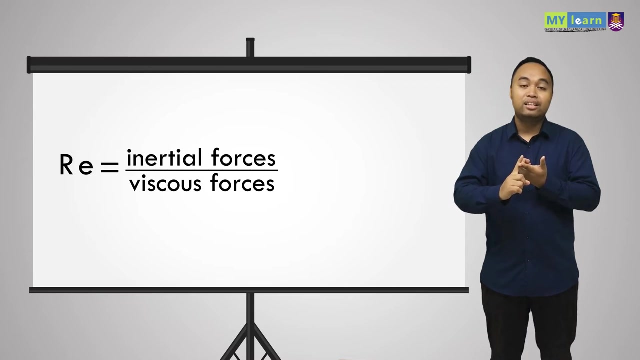 or turbulent, and it is done using Reynolds number, And Reynolds number actually comes from Oswald Reynolds, so you know why it's called as Reynolds number, And it is discovered around 1880s. It is actually a ratio of initial forces and also viscous forces, And it is 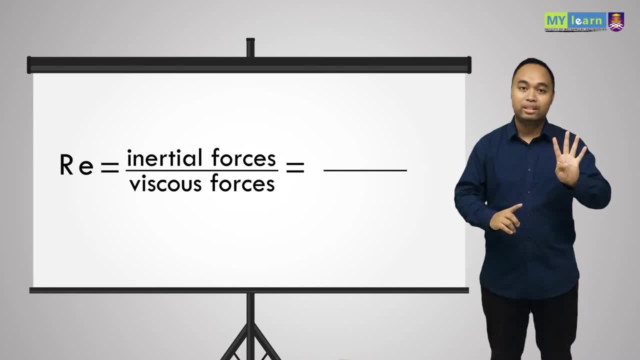 actually been calculated through four different parameters, And the first parameter is the density of the fluid. The second parameter is the velocity of the fluid, The third one is the characteristic length of the pipe And the last one is the dynamic viscosity of the fluid. The calculations on Reynolds number will be shown in the video later. 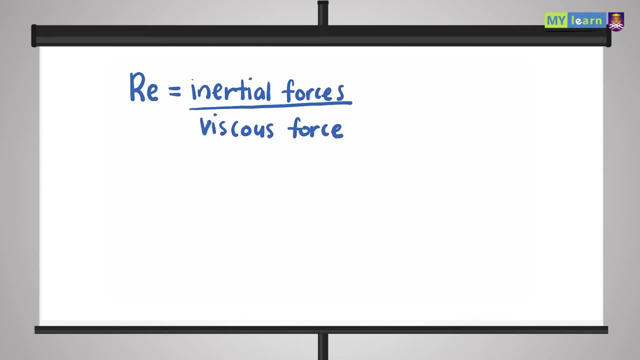 Hello everyone, welcome back to our study on Reynolds number. So for this video, we will teach you how to calculate the Reynolds number And also we will decide whether a flow condition is a fluid or a fluid. So let's get started. 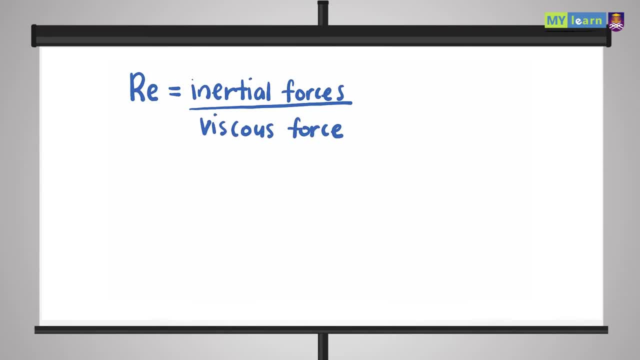 So the flow condition is laminar, turbulent or transitional, based on the Reynolds number that we get. Okay, Reynolds number is actually a ratio between initial forces and also viscous force, And for the initial forces it is highly affected by the velocity of the fluid inside. 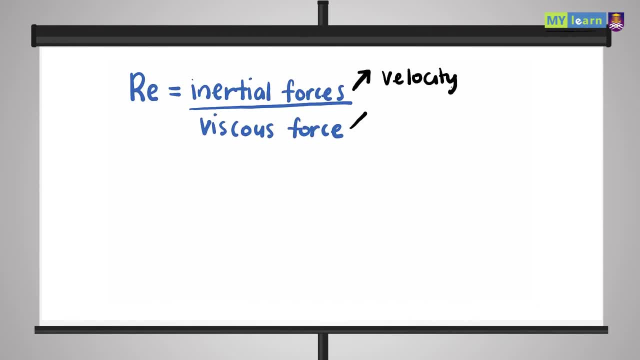 the pipe, While for viscous force it is highly affected by the stickiness of the fluid. all we call it as dynamic viscosity. So seeing from this condition, we know that if the velocity of the fluid is much higher, the Reynolds number will increase, And also if the viscous 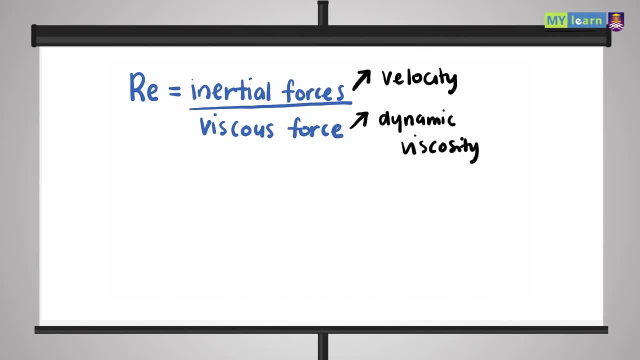 force is much lower, the Reynolds number will also increase, Because when you have less stickiness or viscosity, it means that the fluid can move through the pipe much smoother and much faster. So how do we calculate Reynolds number? So Reynolds number is equal to rho V, D over mu. 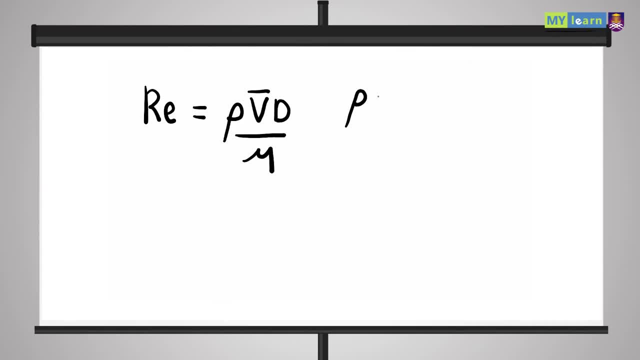 The rho is actually the density of the fluid, The V is the velocity of the fluid, And the velocity of the fluid is the density of the fluid. And for the D it is actually the characteristic length. And for our study, since we are using pipe, we are actually using D, which is the 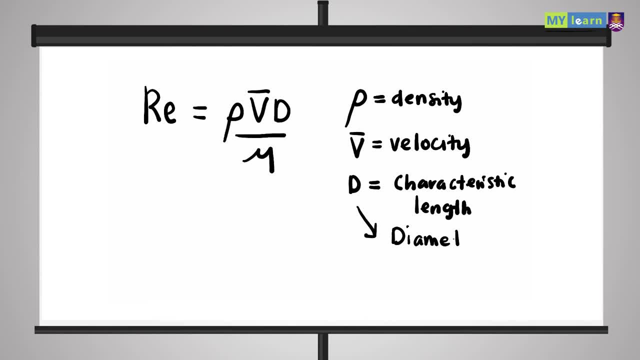 diameter of the pipe. Once the浅 means the velocity large in diameter, once the Mu means the viscosity large in diameter, then we are absolutely talking about IK/ Now, when Ray Zetford asked us to calculate the ρ, we got upward. protein density of the. 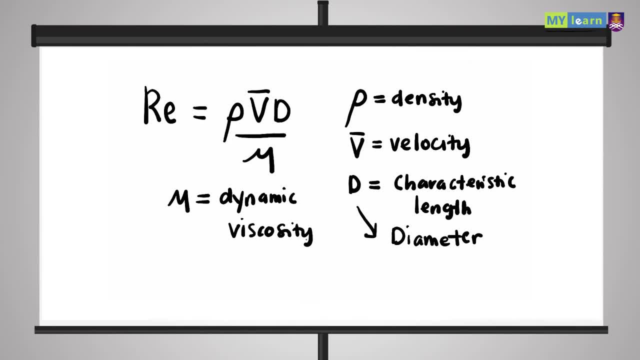 fluid. So you can see here his program is somehow when the rated parameter this. instead of so, Let us calculate the v essay, which says it is when the rated parameter of the fluid is x2.. So it is x2.. The slighity time we should sets just below 0. 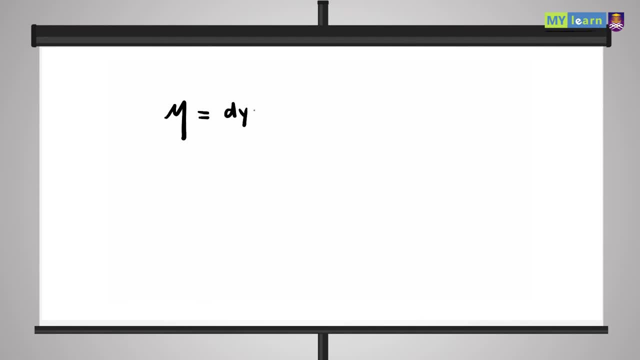 Press F to Al inteligens, which is dynamic viscosity, if we be dividing it with density, will equal to kinematic viscosity. so kinematic viscosity, okay, can be used in the Reynolds number by changing the Reynolds number into this equation. okay, to simplify this, we can either put Reynolds number to be rho, V, D. 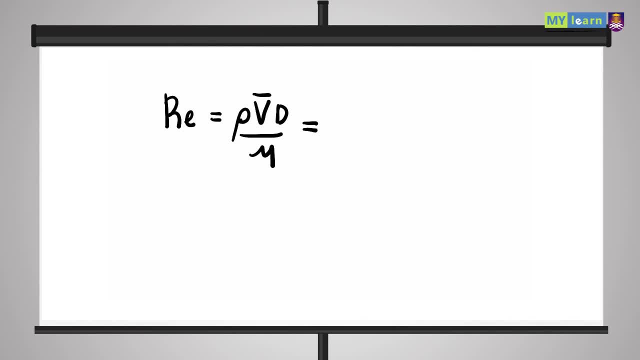 over mu, or it is also equal to V D over kinematic viscosity. okay, since both the top and the bottom part of our equation is forces, so it means that the unit will be the same. so for this particular equation, Reynolds number is dimensionless, meaning we don't have any unit for Reynolds. okay, so what is the important? 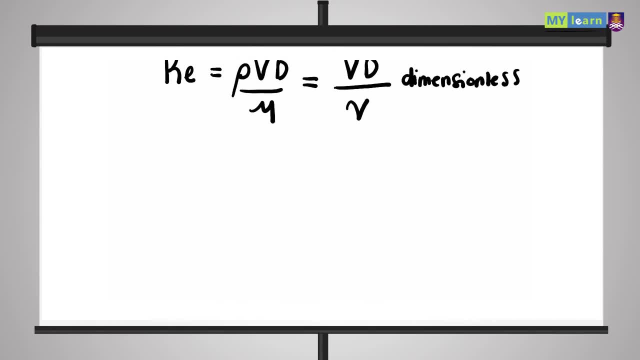 of Reynolds number to our study. so in order for us to know whether the flow is laminar, turbulent or transitional, we have to know the RA critical of the study. so RA critical is a number which represents the condition when laminar becomes turbulent. so for piping system the RA critical is equal to two thousand three hundred. so for piping system the RE critical is equal to two thousand three hundred. 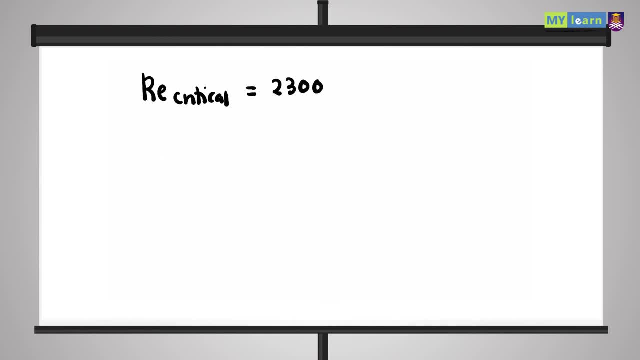 so because of that, if you have RE lower than propriately than the flow can be considered as laminar. if the re is in between two thousand three hundred and four thousand, to get amylamericARD equal toか- with respect to flow as well, Valolable per cachet can be considered laminar. if Pause for a moment. 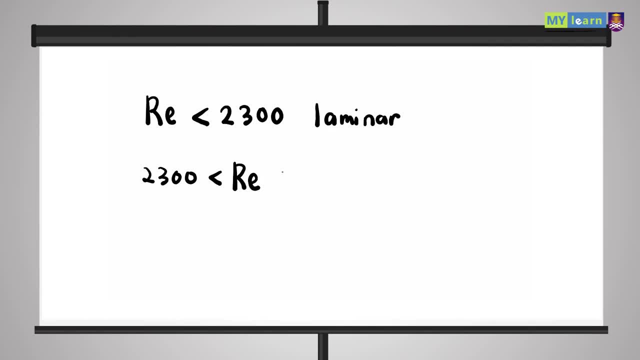 2,300 and 4,000, the flow is considered to be transitional, which means the flow is fluctuating between laminar and turbulent, while if the Re is higher, the same as 4,000, the flow will be turbulent. however, for the purpose of our study, 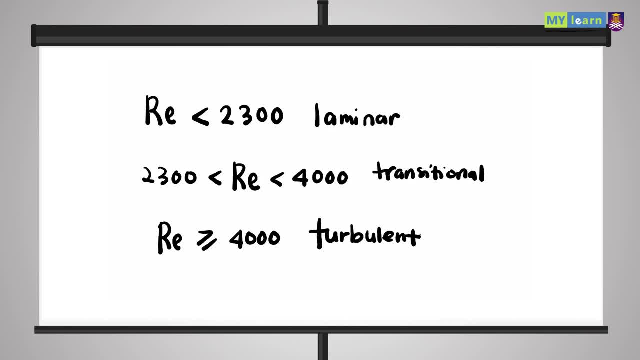 we only consider laminar and turbulent calculation and we don't consider transitional calculation because it is much more complicated. so what we can say right now is: for our purpose, in MAC 241, if the Re is lower than 2,300, we consider it to be laminar. 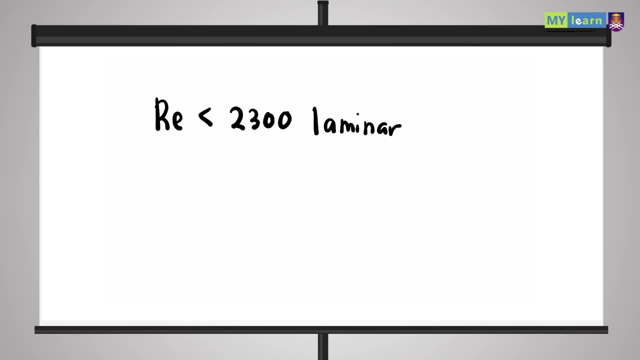 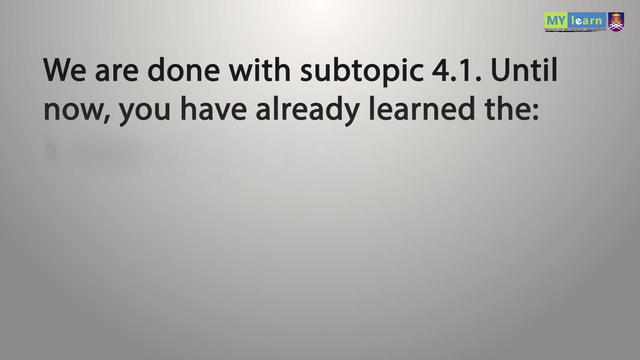 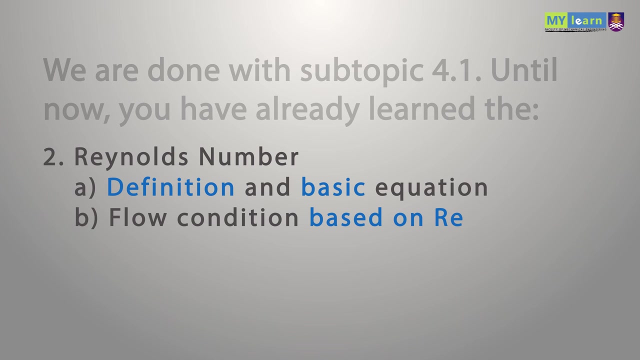 and if the Re is bigger or the same as 2,300, we can consider it to be turbulent. okay, I think that covers out the calculation for Reynolds number and hope to see you again later. so till then I'm Sham good luck and bye, bye you.